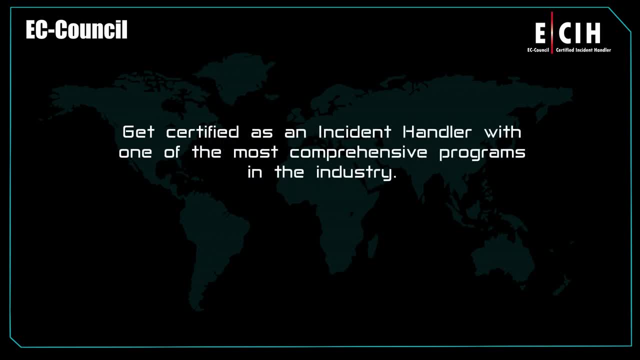 Get certified as an incident handler with one of the most comprehensive programs in the industry: 16-plus job roles, 10,000-plus job openings, average salary of $91,385.. To know more, visit EC Council Certified Incident Handler program. wwweccgov. 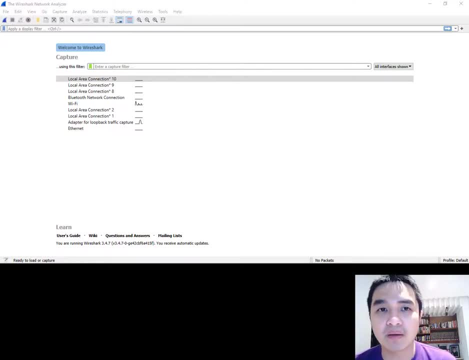 Okay, so most of the videos I published were how to design a network, but we do also need a video on the tools needed to debug or find problems in existing networks. Okay, so I'm going to talk about two tools here. The first will be Wireshark. This allows me to analyze the packets that I can. 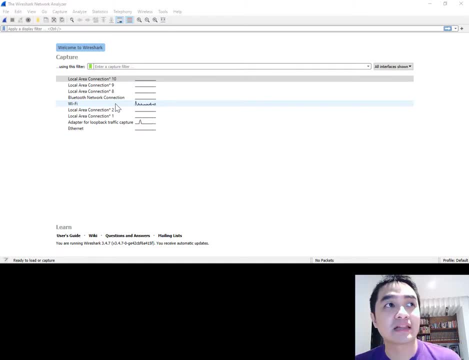 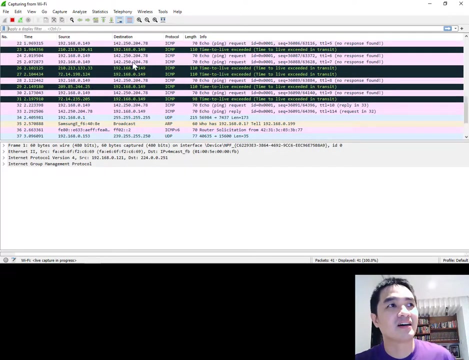 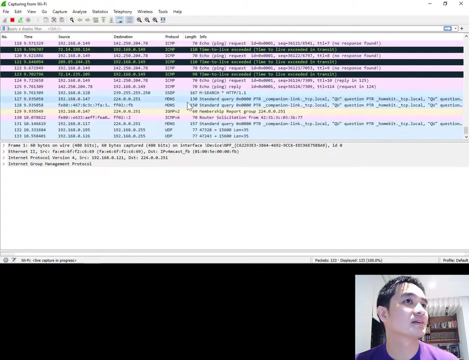 see on my device. So here I'm connected on my laptop and I can analyze things on my Ethernet card and on my Wi-Fi. So I'm going to click Wi-Fi And by doing that I'll see all the traffic on my network And here we can actually see the probable bad packets And look. 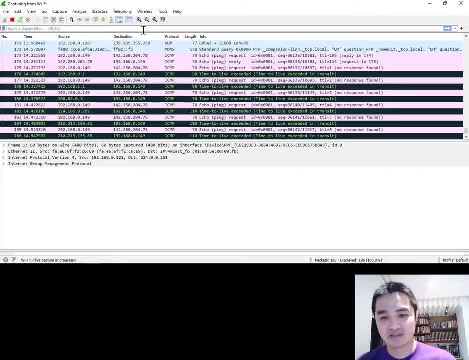 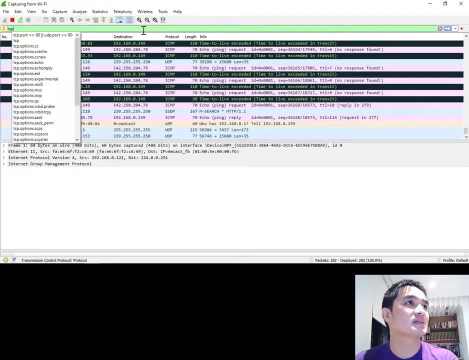 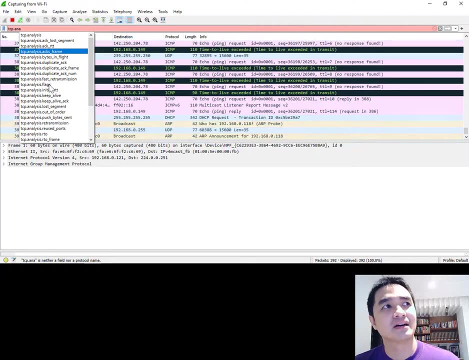 all of this time to live exceeded stuff. So what we can do is we can actually do things like say we can do TCP dot analyze, analysis, dot flag. This will actually give us all the TCP packets on my network that are having problems. 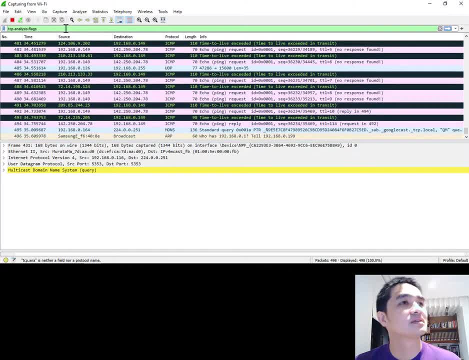 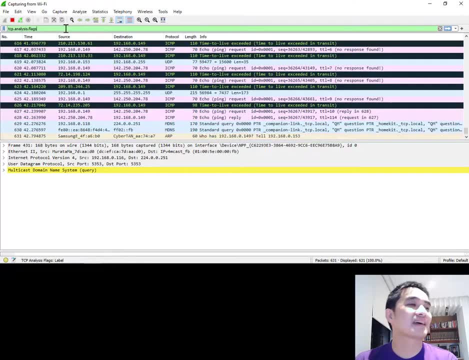 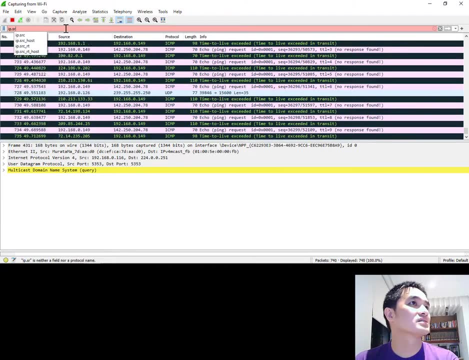 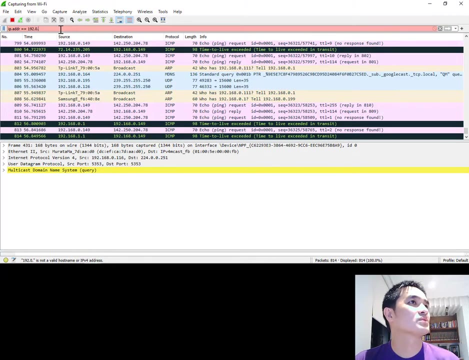 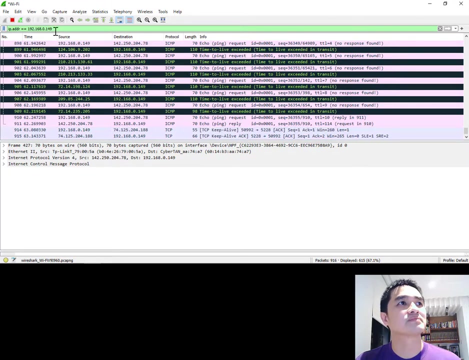 And we can see: okay, so these are the ones having problems, And it's a lot. And then I can do things like: and then I can add more things. or I can say IP, dot source equals dot source, address equals 192.168.0.149, and then I'll only get things.